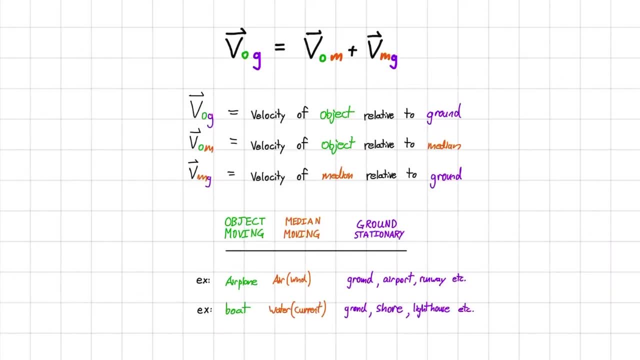 So in this video I'm just going to walk through a quick introduction to relative velocity in two dimensions. So here we have an equation that we're going to use quite often, That's the velocity of the object relative to the ground is equal to the velocity of the object relative to the median. 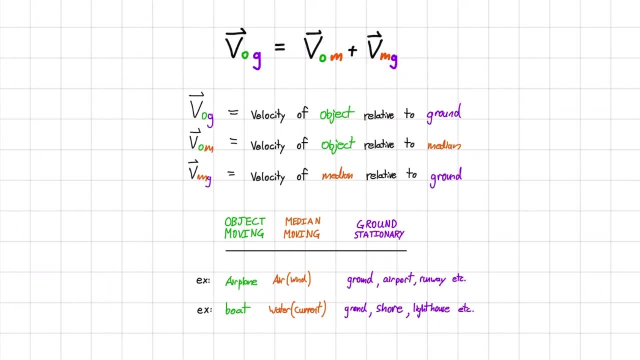 plus the velocity of the median relative to the ground. And if you see, here I have these written out and color-coded so it's clear and easy for you to follow along. And then at the bottom here I have some examples of some common problems that we'll see. 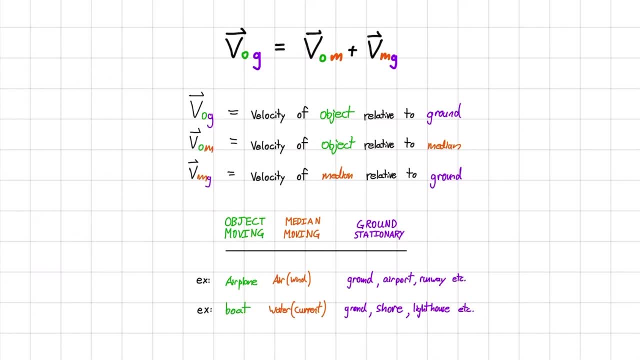 So with the object, it's always going to be something that's moving, and in common and common problems you'll see that as either airplane or a boat. And then for the median, this is the median in which the object is moving, but the median itself is also moving. 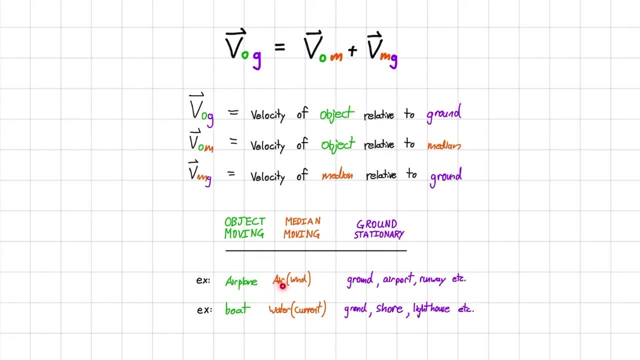 So this is the median in which the object is moving, but the median itself is also moving. So examples of these: with airplanes you'll often see the air or a certain wind, So the airplane is flying in the wind, but the wind is also moving. And then with the boat example. 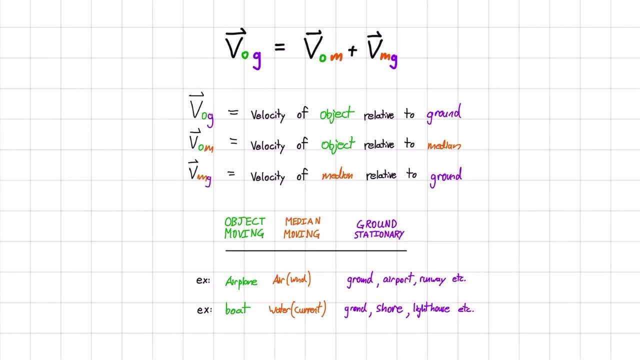 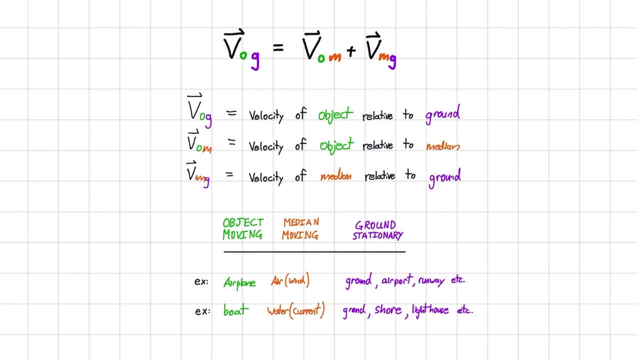 you'll often see it with water or a current, So the boat is traveling a certain speed in the water, but then the water or the current also has a certain speed, And then for the ground you'll see, this is the part that we define as stationary, Although the ground is actually. 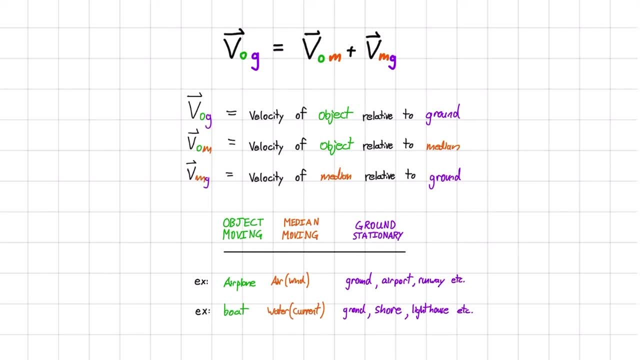 moving because the surface of the earth is moving through space. we define this is what we define to have a velocity of zero. So it is, we define it to be stationary. So in these examples the airplane will either be the ground or the airport or a runway, or it might be some landmark. And then with the boat example, 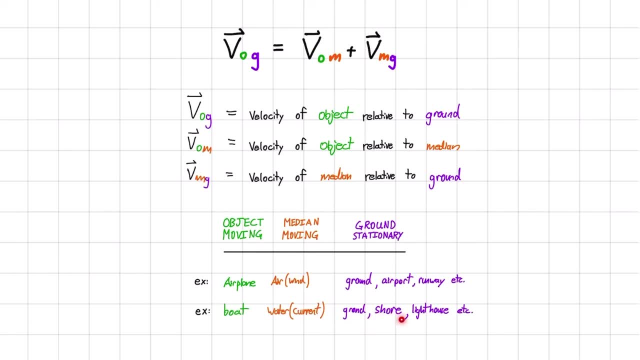 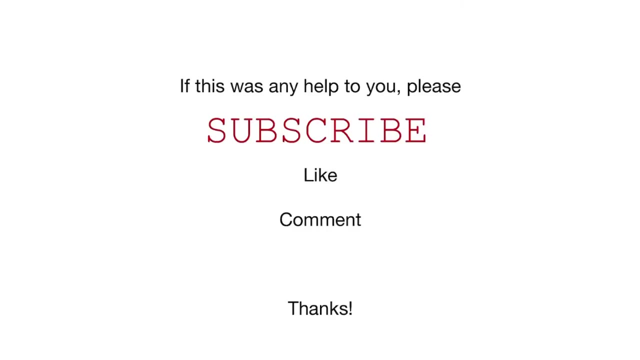 example, you'll often see the shore as a stationary or a lighthouse or something along those lines. So that's it for this introductory video. If you want to see some examples, you'll be able to find more on this channel.